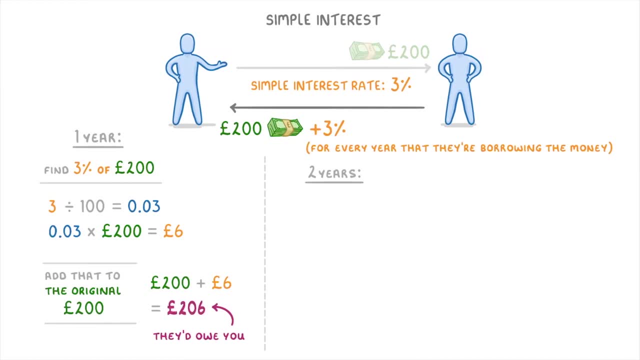 For this we could just take how much they'd owe you after one year, so the £206, and then add on another year's worth of interest, so add £6, which would bring the total debt to £212.. This technique is pretty good. 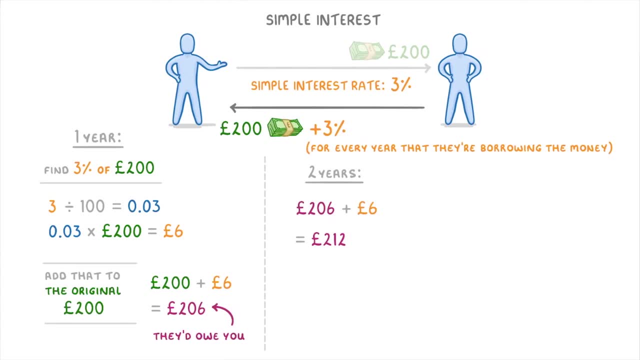 if you just have very low numbers, so one year, two years, three years and so on. But if they ask for a much longer period, like 10 years, then we might need to use a slightly different technique. For this we could still take the original £200, but this time we'd need 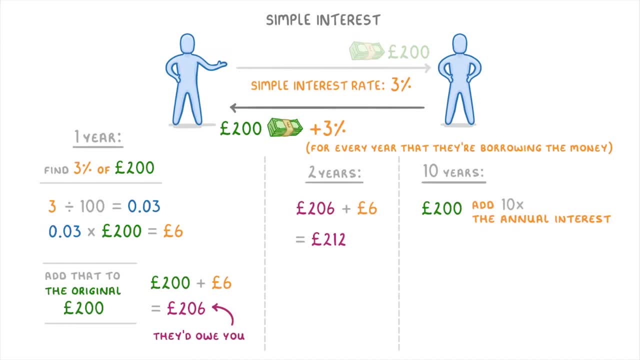 to add 10 times the annual interest because they're borrowing it for 10 years. So £200 plus 10 times £6, because it's going to be an extra £6 of interest each year. So that gives us £200 plus £60, or £260 in total. 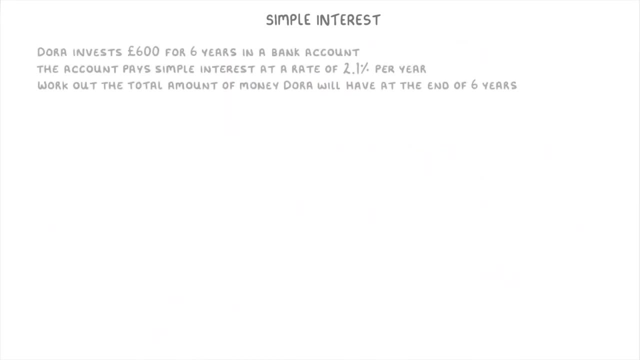 Let's try another one and give the video a pause if you want to give it a go first. So in this question we're told that a drawer invests £600 for 6 years in a bank account and that the account pays simple interest at a rate of 2.1% per year. Our job is to understand how that works, So let's try this again. So we're told that Dora invests £600 for 6 years in a bank account and that the account pays simple interest at a rate of 2.1% per year. 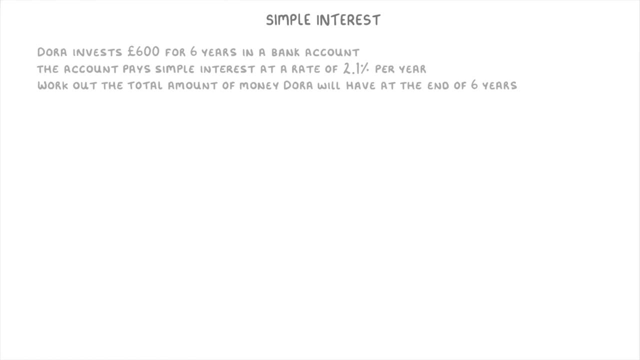 work out the total amount of money that she'll have at the end of the six years. So for this one we need to take the £600 original investment, because you'll get that back at the end, and add six years worth of annual interest, And remember to work out the annual interest we just 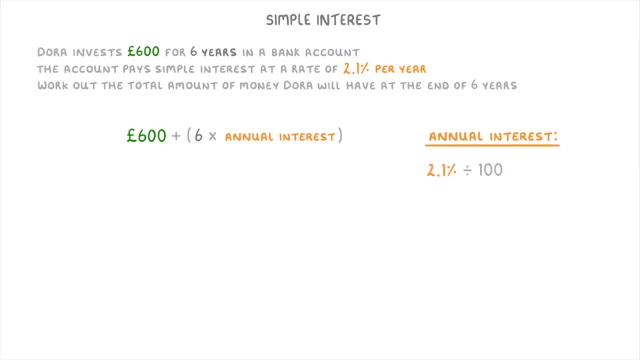 convert the 2.1% to a decimal by dividing it by 100,, which would be 0.021, and then multiply it by the original amount of £600.. So that would give us £12.60 of interest each year. 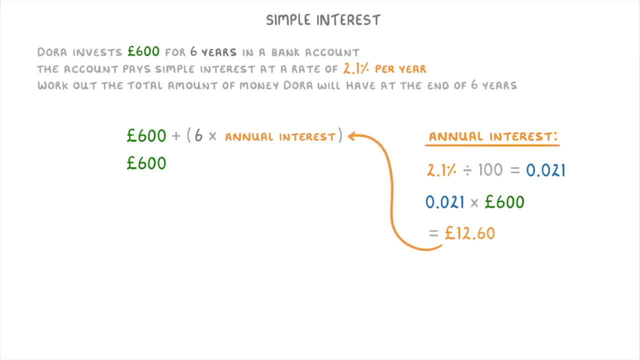 Then if we substitute this into our equation, we get £600 plus 6 times £12.60. And so if we simplify that, that gives us £600 plus £75.60, and so a total of £675.60. Anyway, 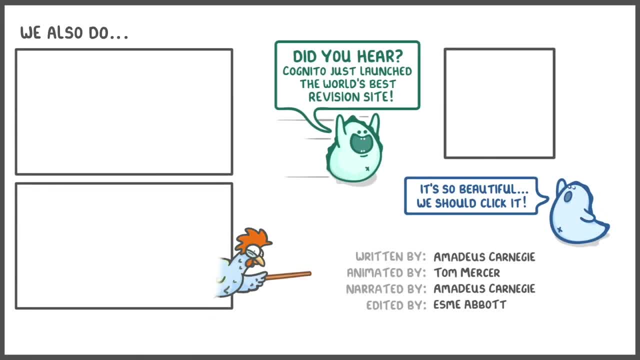 that's everything for this video, so I hope that made sense. If you liked it, then please do give us a like and subscribe, and we'll see you again soon. Cheers.